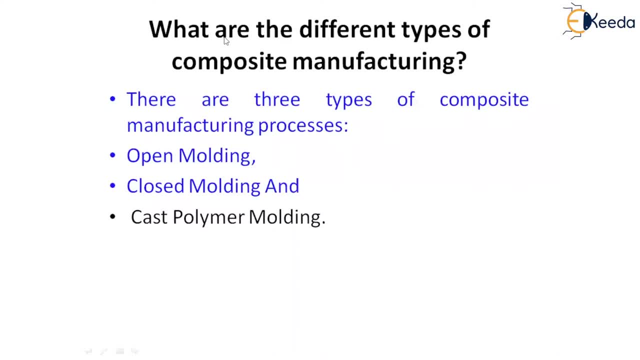 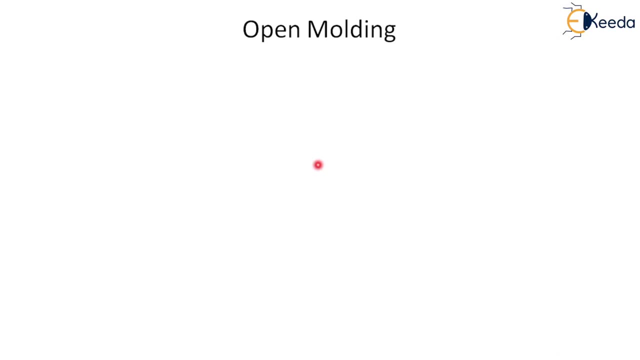 which are available in producing the composite manufacturing. Now let me discuss the each and every molding process in detail. First of all, we will start with the open molding process. So what is exactly the open molding process? what we are doing in open molding process, In open molding process? 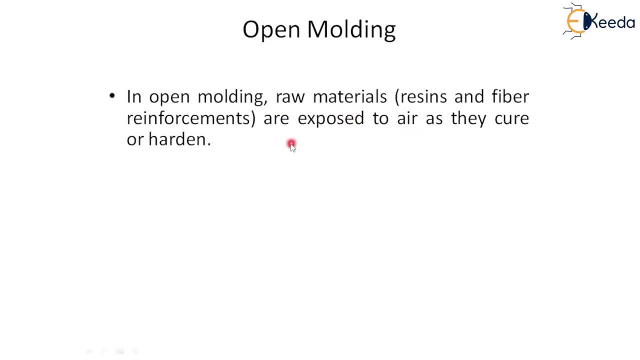 in general, raw material is exposed to air, So that means during the process it may be curing or it may be hardening process or whatever the process is happened in open molding process. In this open molding process the raw materials are exposed to air. So that is one particular that is important. 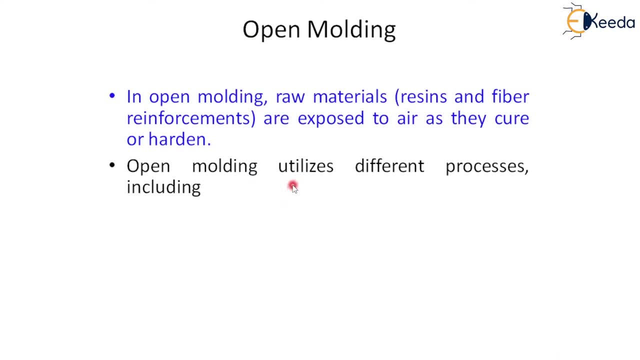 point in understanding open molding, and it utilizes the different processes, including hand layoff method. That means this is the one open molding process and another process is a sprayer. So this is the one open molding process and another one is casting and filament winding. 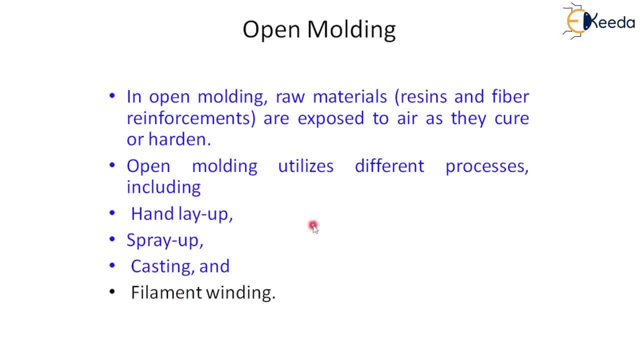 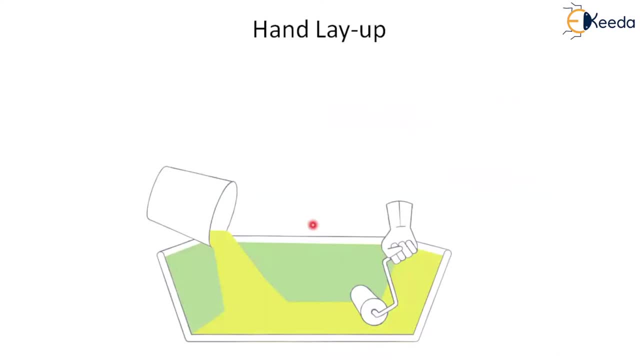 So these are the various open molding process which are utilized by the people, and the process is also very simple. So let me start with one example, that is, hand layoff method. If you see the image here, this particular image shows a simple equipment in which the 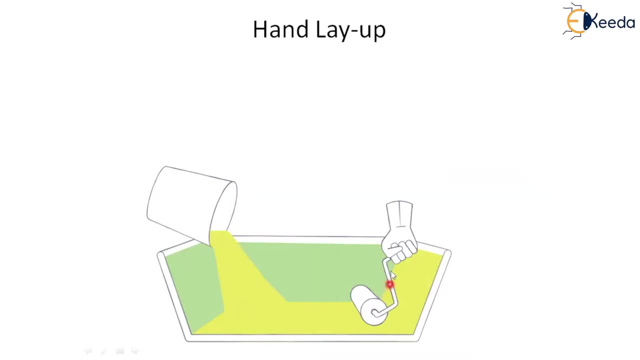 resin. the material is poured here. Here, the pressure roller- this is a pressure roller- is a available. with help of pressure roller, we are applying the pressure on the materials. Now what we are doing in hand layoff method. So it is a very, very cheap and expensive method. That is the least. 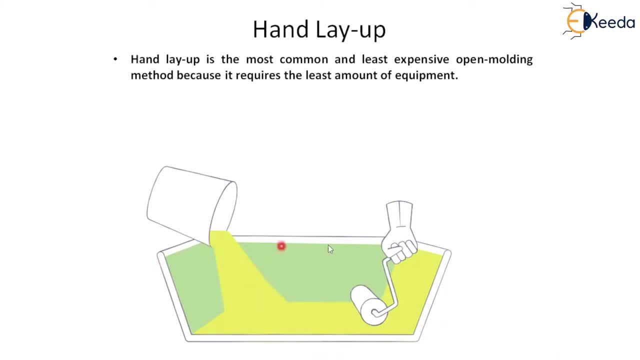 expensive in open molding method because it requires the least amount of equipment. The equipment which is utilized in hand layoff method is very, very low in cost, So that's why it is a cheaper method compared to the other manufacturing process And the fiber reinforcement are placed. 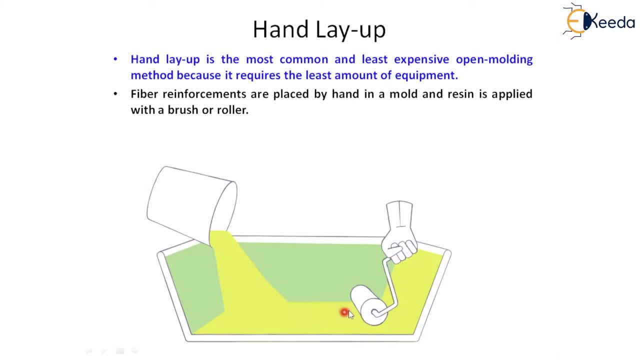 by hand. only that is in a mold, and the process is very simple. So that is why it is a cheaper method compared to the other manufacturing process. And the fiber reinforcement are placed by hand. only that is in a mold. resin is applied again with a brush or roller, So that means in first coating. 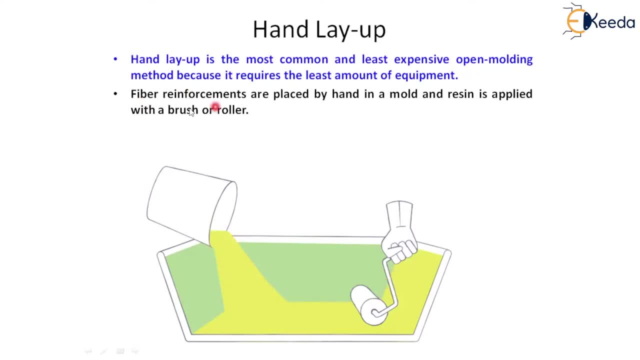 first of all, resin is applied in second, coating, the fiber reinforcement are placed at various positions and after that, again, resin is applied with a brush or roller. The process: what are the process that we are utilizing here? this is used. there is a hand up method can be. 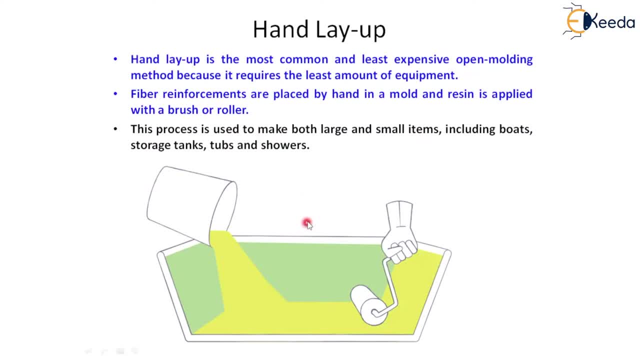 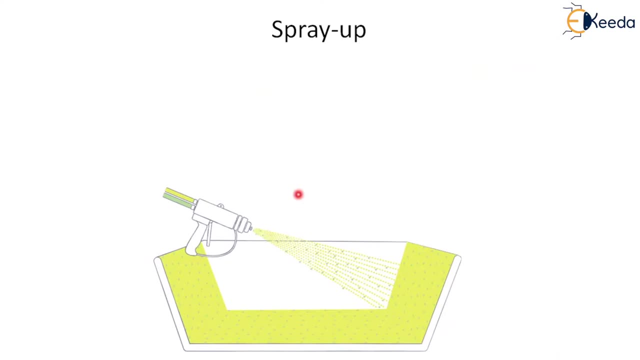 utilized to make both large and small items, including boats, But these boats can be manufactured. tanks, storage tanks can be manufactured, tubes can be manufactured. showers can be manufactured with help of a hand layoff method. If you see the another method, the only change is the equipment in 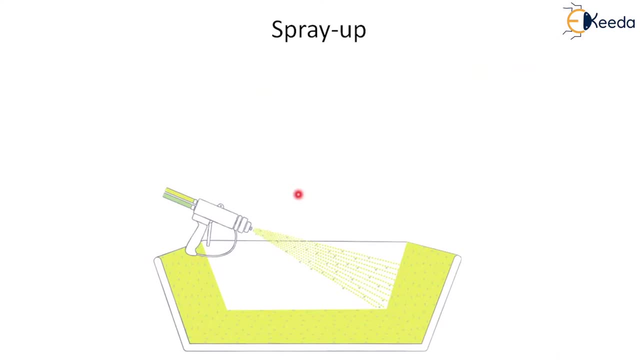 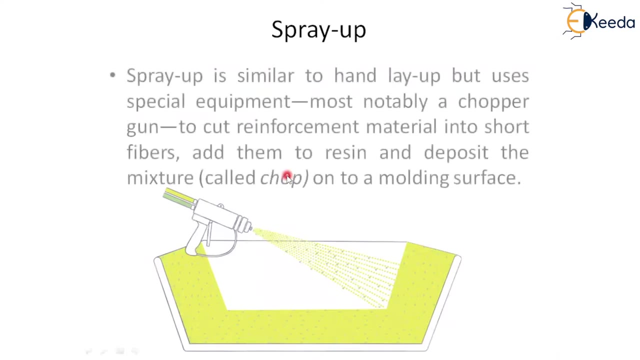 which methodology you are applying the material. So that is the only change. the remaining equipment, everything is the same. there is a spray up method. So that means here we have to take the torch gun or a spray of method, that is, which is with which we can spray the raw material directly. 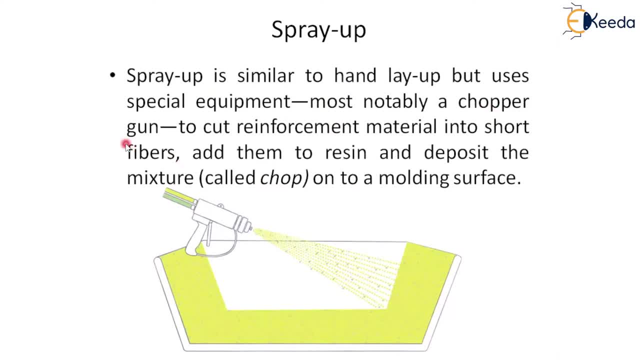 onto the surface. That means most notably chopper gun to cut the required material into short fibers and then to resin and deposit the mixture onto a molding surface. That means here this buttless sprayer method is just giving the uniform molding process, which is not possible manually. This is the 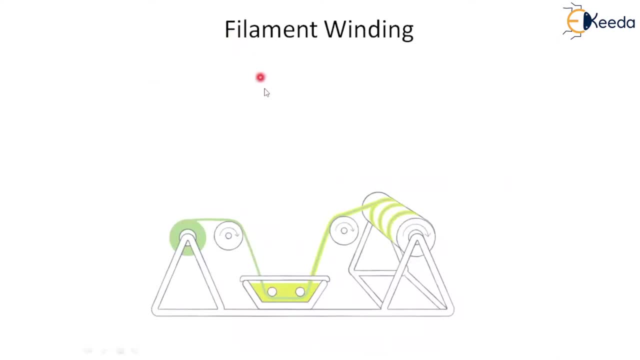 second method and the next method is filament winding. So in filament winding, if you observe here, it is an automated process. Filament winding, This is an automated process That means the rollers will move automatically with the help of some power rollers and that applies a resin saturated continuous strands Here. what 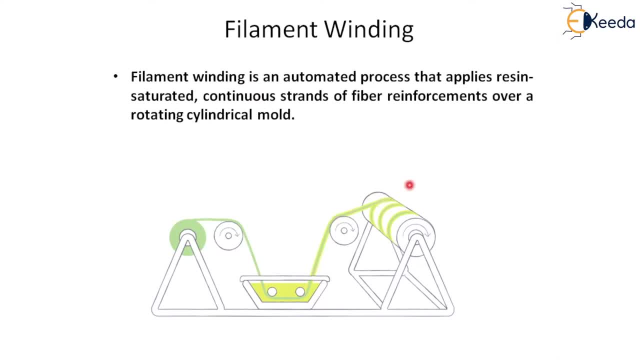 is required is continuous strands of fiber reinforcement over a rotating cylindrical mold. I repeat here: to operate this system, continuous strands are required and the fiber is reinforced continuously over a rolling cylindrical mold. This has happened in flat diamond welding, but in general it is used for hollow products Like rocket monitor casing, pipe stacks and the chemical Ol園can. This is the various methods are available: inlex and 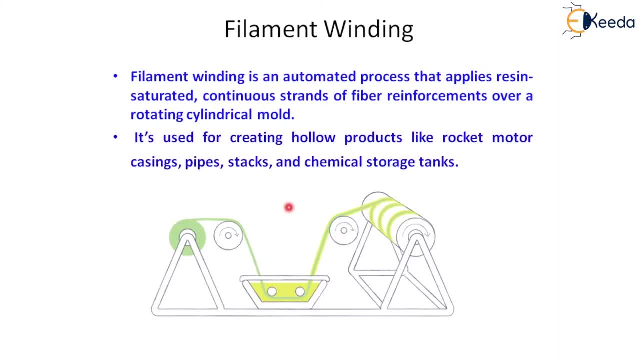 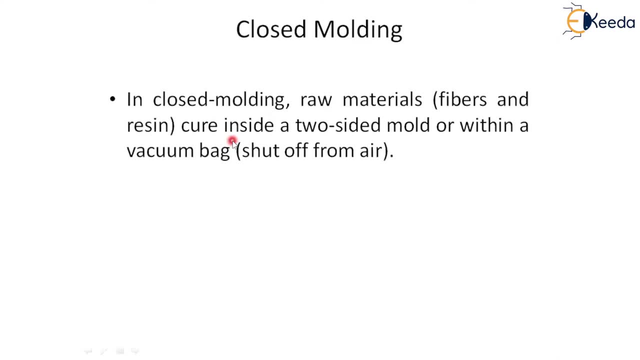 producing composite materials. Here this represent as a filament winding In close molding. raw materials in close molding. here Customized raw materials are cured inside a two shielded hull model- there is two shielded uh mold- or within a vacuum bag. so here the important parameter is raw. 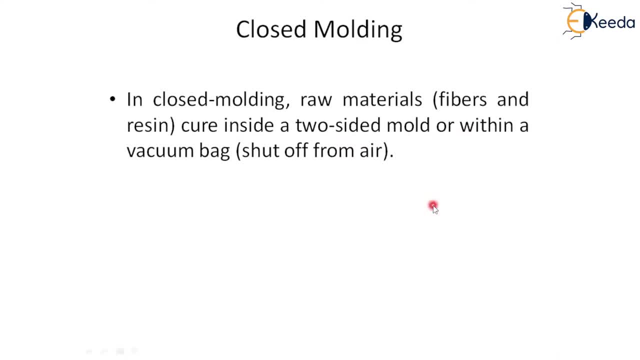 materials inside the mold or within the vacuum bag. so that is happening. closed molding process and closed molding process are usually automated and require special equipment, so they are mainly used in large plants only, not in small plants, for each and every small plant cannot be designed for the new equipment. we have to analyze, we have to test that particular model properly generally. 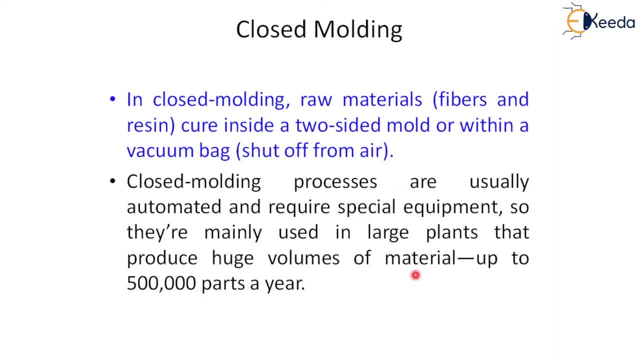 we can understand that, whether that model is giving a proper guidance or not, and there are many used in large plants that produces huge volumes the material, which you can say that up to almost five lakhs parts per year. so this is happening, close cold. that is a closed molding. 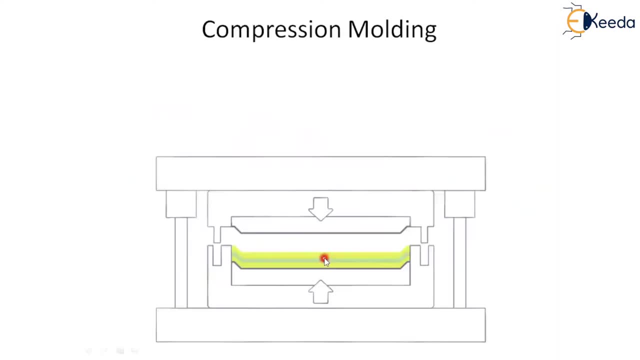 process. now let me discuss the other process in the hand layup method, that is, the compression molding. if you see the image- see the image here is a compression from two sides. we are trying to apply the pressure because one plate is fixed, other plate is moving, and this particular manufacturing process in which composite materials are sandwiched, 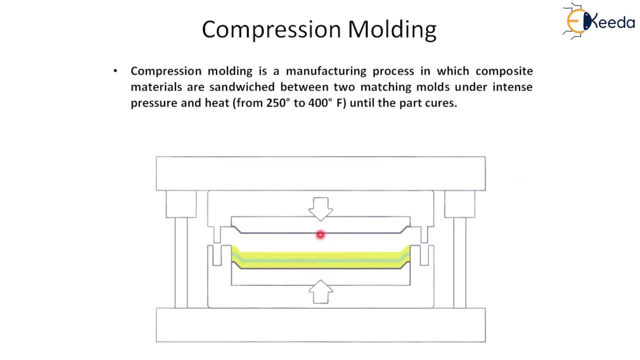 between two matching, that is, molds under intense pressure and the heat 250 to 400 degrees centigrade until the the part pressures. here the temperature is important in compression molding at what temperature you are giving the heat to the material or you are doing the process to the material. here you can say that this technique is used generally to rapid. 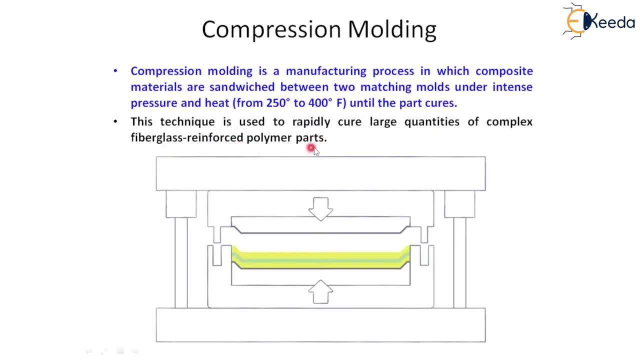 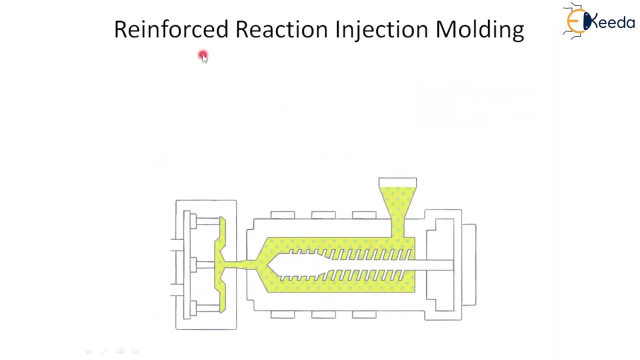 pure large quantities of complex fiberglass reinforced polymer part. so here the technique is important. and what are the equipment? the equipment is very simple, just, it is applying compression on the material so that we can check the fracture strength of the material. and if it is material, sometimes it is very difficult to break, it is difficult to apply the load also. now come to 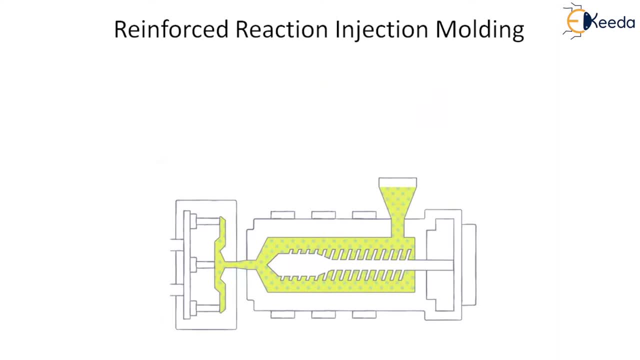 the point here- a rain force reaction injection molding. so whenever the rain force reaction injection mode- the name itself is giving that, it is an injection holding and in this injection molding rain force that is attached. rain force is attached, that means the secondary material is attached. see the image here. 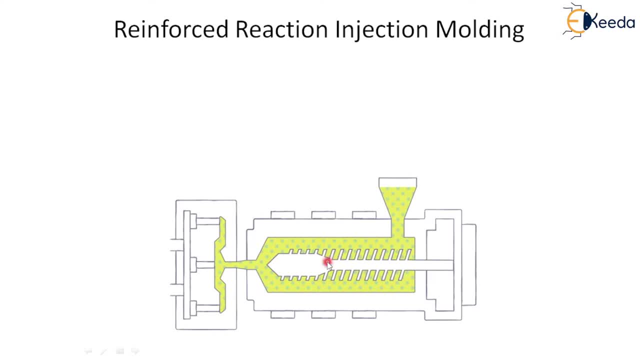 see the image. so this image is having a lot of information. and here the, that is reinforced reaction injection molding is widely used here to make external and internal automotive parts. see here, this is the die. so here for this die the material is forcefully enter, that means with the help of some pressure applied. this is a hopper with which we are pouring. 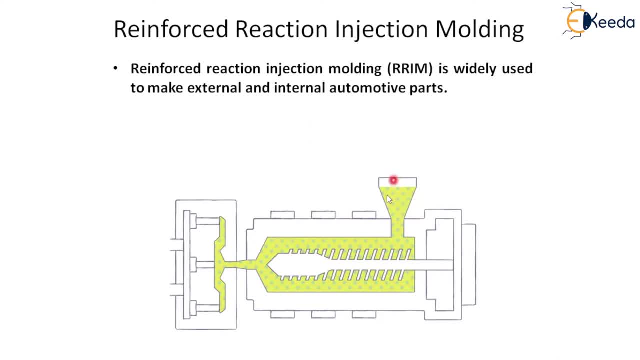 liquid granules or whatever, and these particular hot metal enters into the cylinder. it is like a gun, it acts as a gun and so during this it, like it, will do ball milling process. that means the entire material is going to be crushed anyway. hot metal enters through 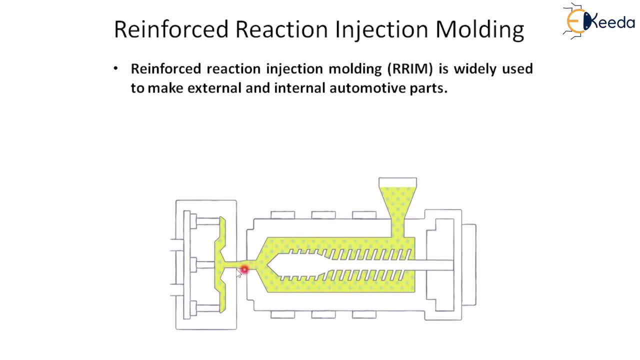 this particular passage forcefully to the die. okay, and you can see the other silent feature of this. in this process, actually, two or more resins are heated separately and combined with milled glass fibers. so that means we can say two resins can be used sometimes, if it is. 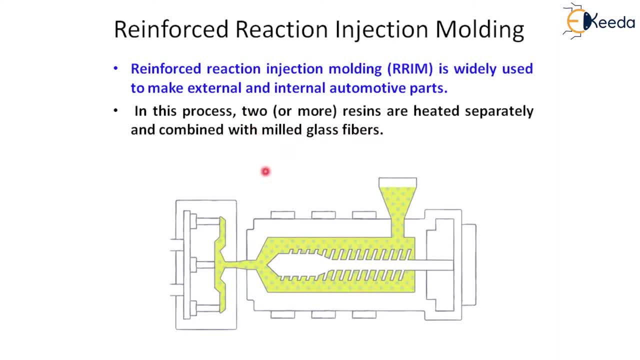 needed only, and one resin is also sufficient to heat the material. now the mixture, whatever the mixture that we are utilizing here, that is, in the hopper, it will mold under high pressure and compressor, so automatically the resin cures quickly and we can get the materials. So this is the process in molding process and that is a closed molding process. 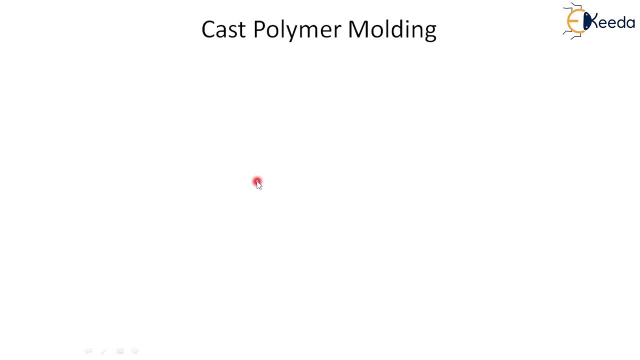 So now another one is cast polymer molding process. What is exactly the cast polymer molding process here? See the mixture: of resin and filler are poured into a mold. So that means in the earlier processes we have poured only the resin, But here in this process we have to pour only the resin, and fillers are poured into a mold. 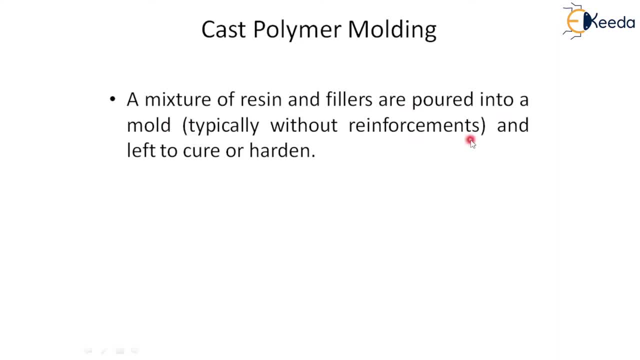 that is typically without reinforcement. That means at this moment, reinforcement is not going to be attached and left to the cure or harden. So this is why this happened in cast polymer molding And the molding methods sometimes use open molding and sometimes use closed molding process. 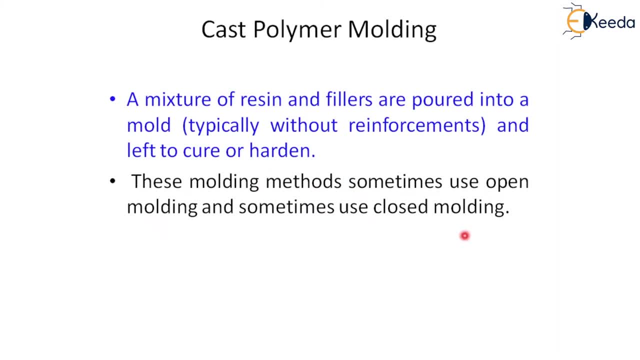 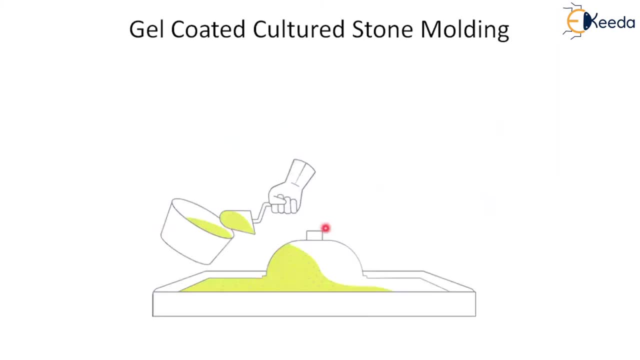 That means these molding methods may not depend on only single process. That is another disadvantage of the composite material And the molding methods see. now let me discuss the other method which is available after the cast, That is, in cast polymer molding gel, coated cultured stone molding process. 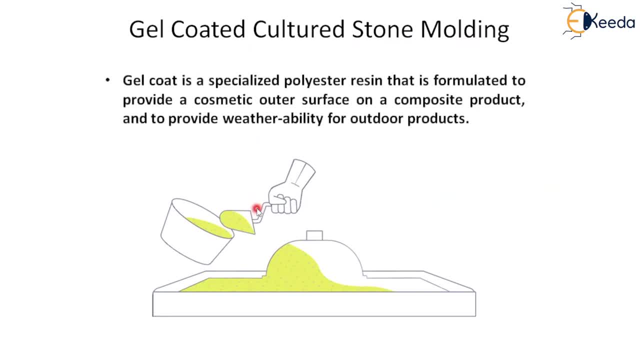 You can see here. first of all, let me explain what is a gel coat? cultured stone molding process, See gel coat is applied first. That is a specialized polyester resin that is formulated to provide a cosmetic outer surface. So that means whatever the outer surface that you want. 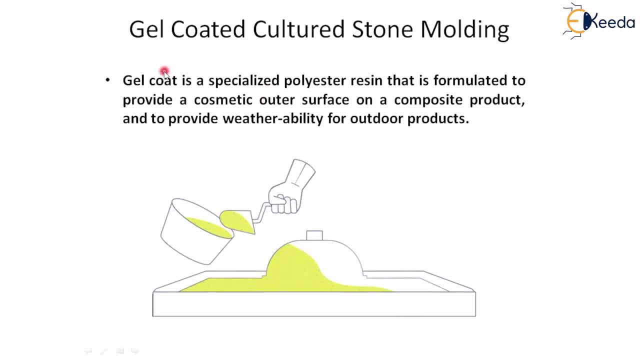 You can do this particular hardening process. That means a gel coated cultured stone molding process on a composite product And to provide whether the ability for outside is outer products or not, See this particular specialized polyester results provides cosmetic outer surface. So that is why this process is very, very important in closed molding process. 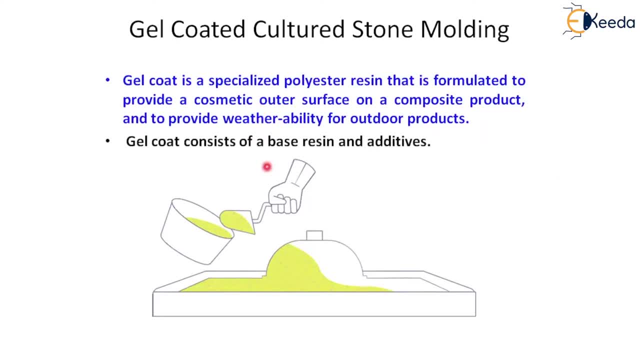 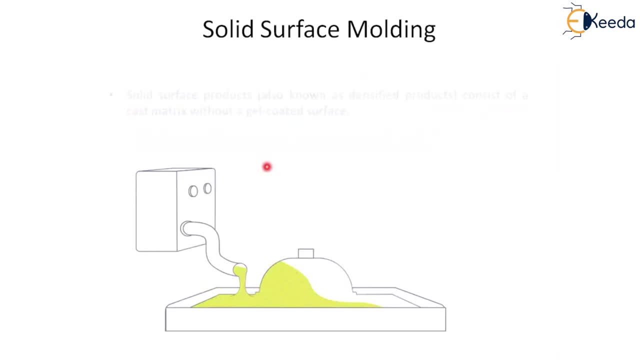 And gel coating Consists of a base resin under edited. now see the solid surface molding. so in the solid surface folding- exactly what happens here- the solid surface products has to be brought and consists of a cast matrix without a gel coated surface. so this is happened in solid surface modeling process and a vacuum can be used to remove entrapped air in the matrix. 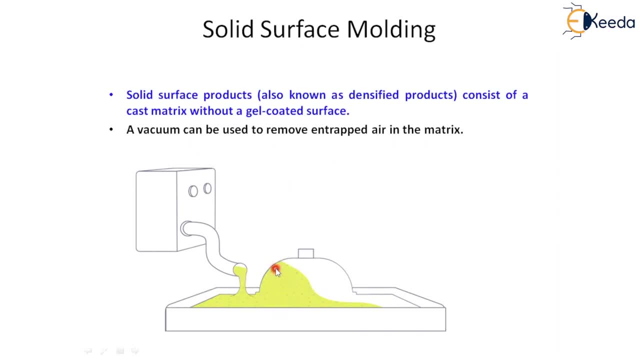 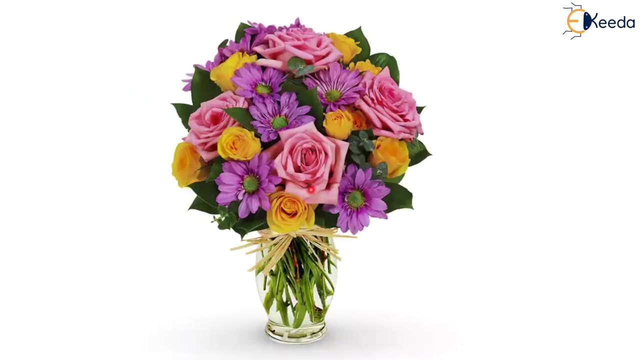 So, whatever the Entrapped air here it must remove, otherwise it will create another problem and it will come out from the failed surface. this is another important parameters, and solid surface products offer limitless design styles and a lot of advantages is here. so this is all about the process and the various processing of composites. in the next coming sessions we will discuss some other technological points. so this is all about processing of coppers. thank you, thank you one and all. Thank you.